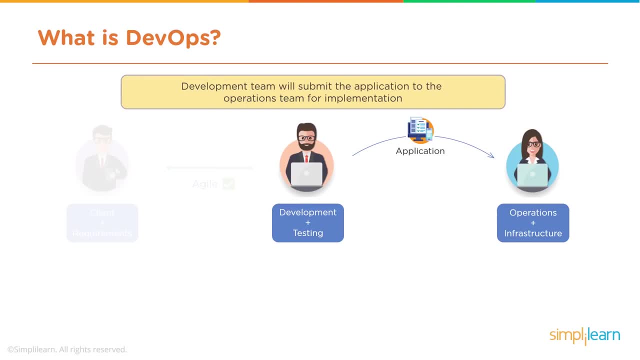 into a single team And they are able to then work more seamlessly together because they are integrated to be able to build out solutions that are being tested in a production-like environment, so that when we actually deploy, we know that the code itself will work. 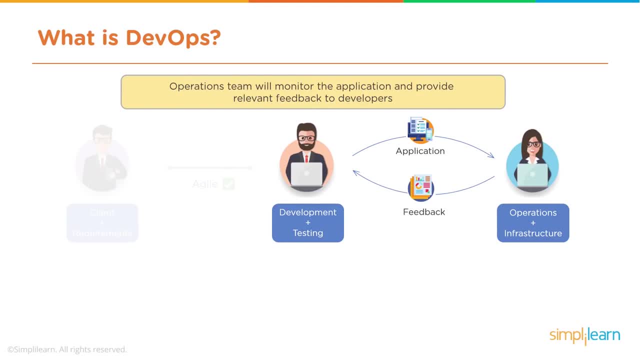 The operations team is then able to focus on what they're really good at, which is analyzing the production environment and being able to provide feedback to the operations team and the development team, And so that's what we're doing, So we're able to work with the developers on what is being successful. So we're able to make 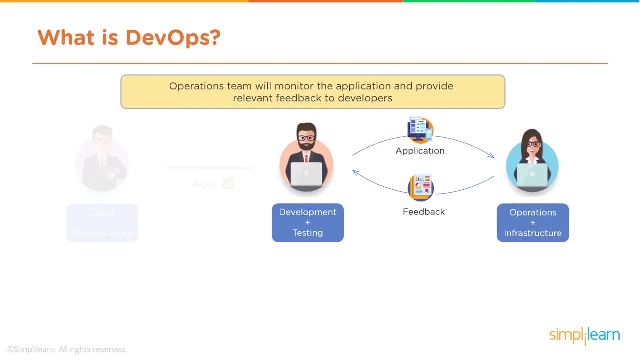 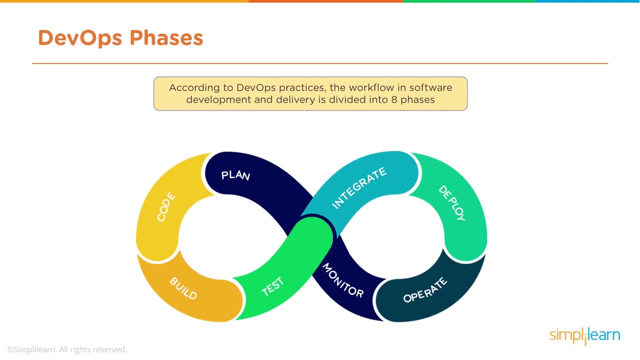 adjustments in our code that is based on data. So let's step through the different phases of a DevOps team. So typically, you'll see that the DevOps team will actually have eight phases. Now this is somewhat similar to Agile, And what I'd like to point out at the time is that, again, 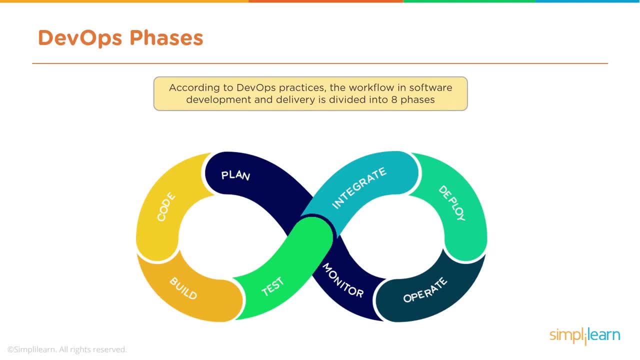 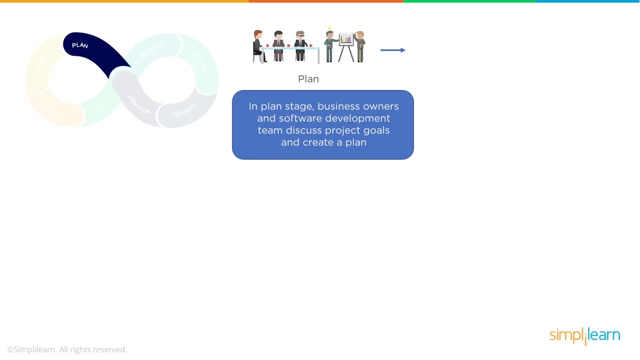 Agile and DevOps are very closely related. that Agile and DevOps are closely related delivery models that you can use With DevOps. it's really just extending that model with the key phases that we have here. So let's step through each of these key phases. So the first phase is planning And this is where we actually sit down. 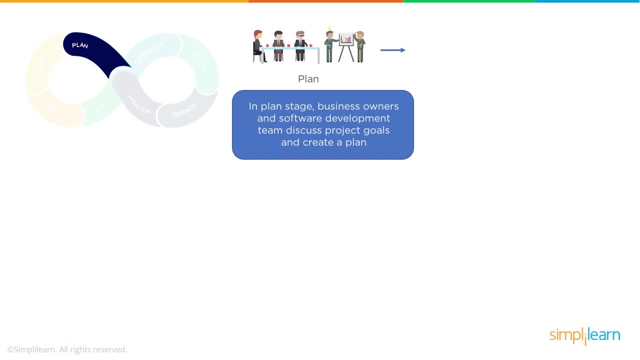 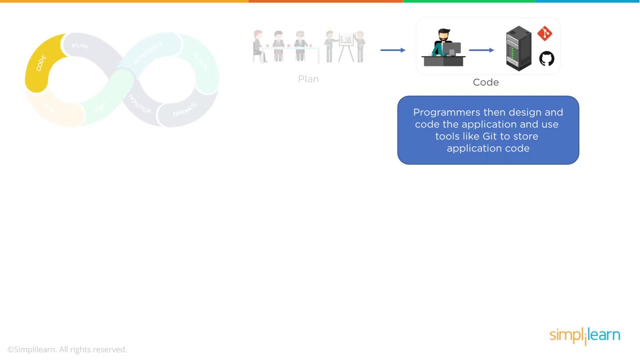 with a business team and we go through and understand what their goals are. The second stage is, as you can imagine, and this is where it's all. very similar to Agile is that the coders actually start coding, But typically they'll start using tools such as. 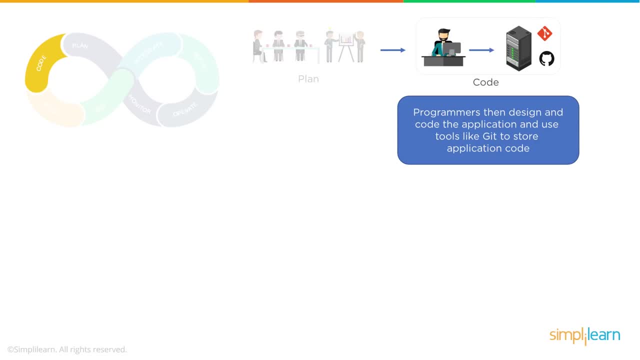 Git, which is a distributed version control software. It makes it easier for developers to all be working on the same code base rather than bits of the code, that is, rather than them working on bits of the code that they are responsible for. So the goal with using tools such as Git is that 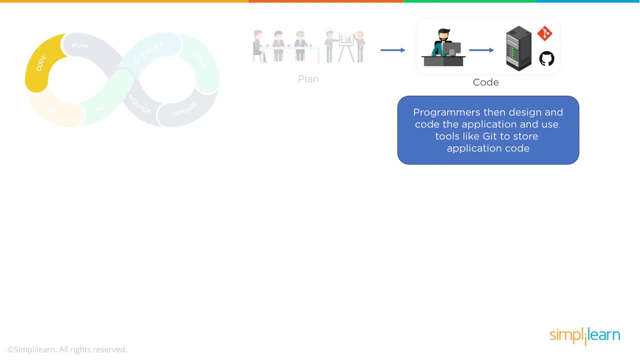 each developer always has the current and latest version of the code. You then use tools such as Maven and Gradle as a way to consistently build out your environment, And then we also use tools to actually automate our testing. Now, what's interesting is when we use 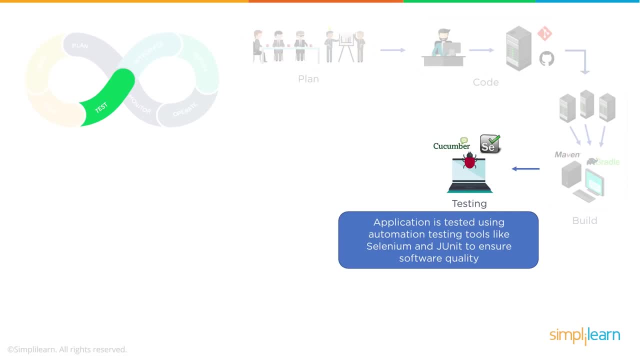 tools like Selenium and JUnit is that we're moving into a world where our testing is scripted, the same as our build environment and the same as using our Git environment. We can start scripting out these environments And so we actually have scripted production environments that we're. 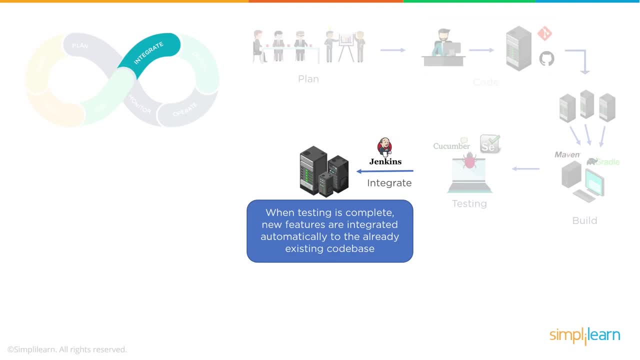 moving towards Jenkins is the integration phase that we use for our tools, And another point here is that the tools that we're listing here, these are all open source tools. These are tools that any team can use, And so we can actually use them to do things, like you know. 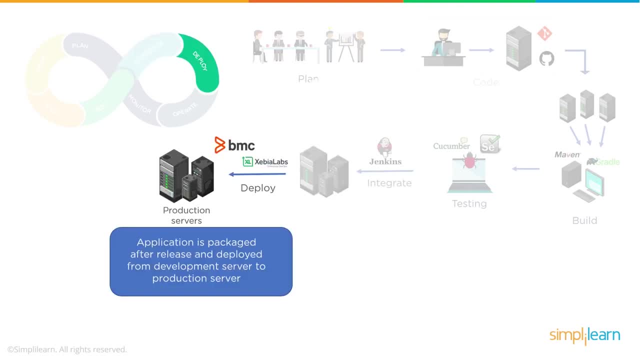 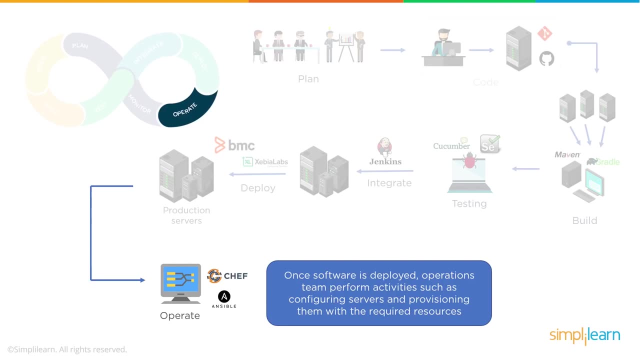 we want to have tools that control and manage the deployment of code into the production environments. And then, finally, tools such as Ansible and Chef will actually operate and manage those production environments so that when code comes to them, that that code is compliant with. 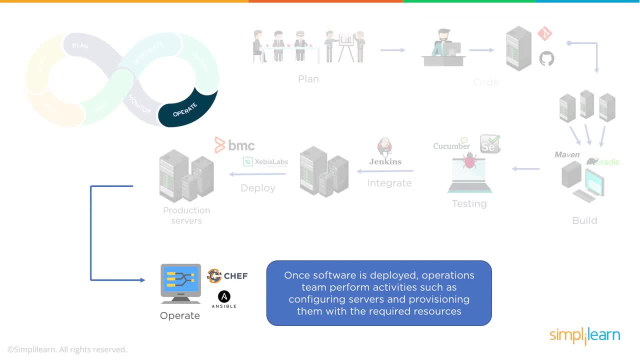 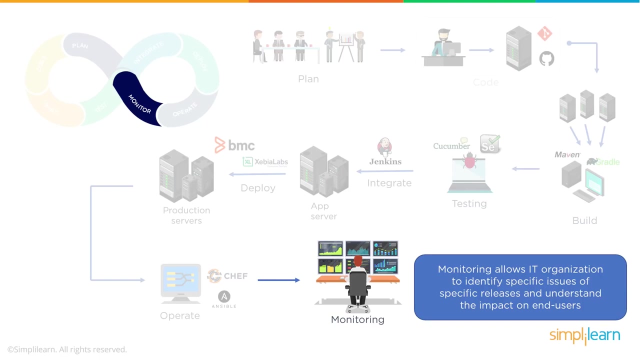 the production environment so that, when the code is then deployed to the many different production servers, that the expected results of those servers, which is, you want them to continue running, is received, And then, finally, you monitor the entire environment so you can actually zero in on spikes and issues. 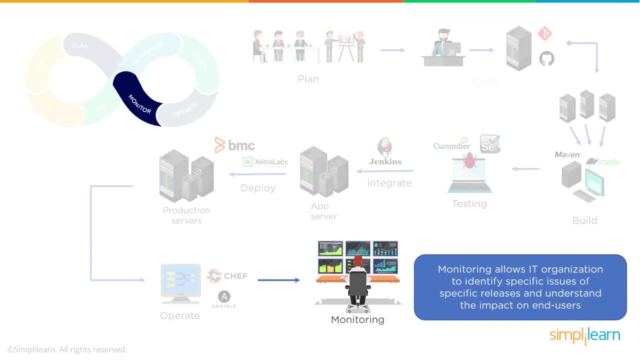 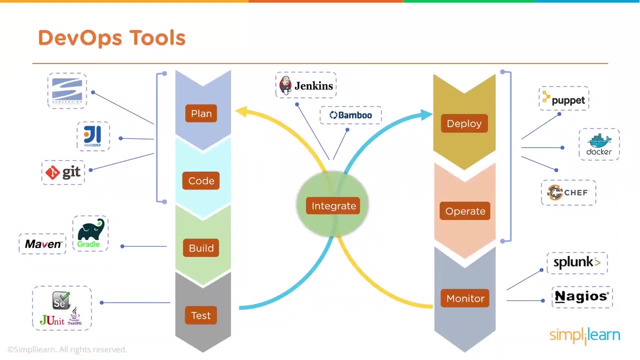 that are relevant to either the code or changing consumer habits on the site. So let's step through some of those tools that we have in the DevOps environment. So here we have is a breakdown of the DevOps tools that we have And again, one of the things I want to point out is that these tools are: 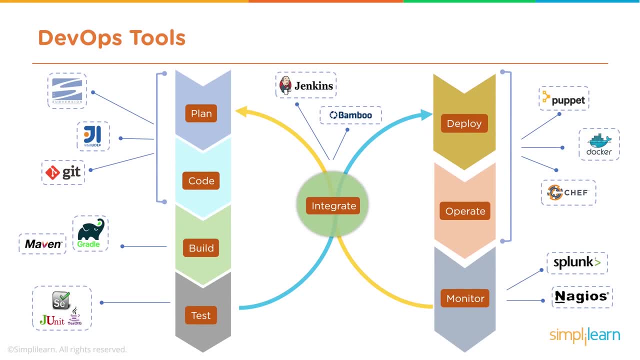 open source tools. There are also many other tools. This is just one of the most common tools that we have And it's really a selection of some of the more popular tools that are being used, But it's quite likely that you're already using some of these tools today. You may already be using Jenkins. You may 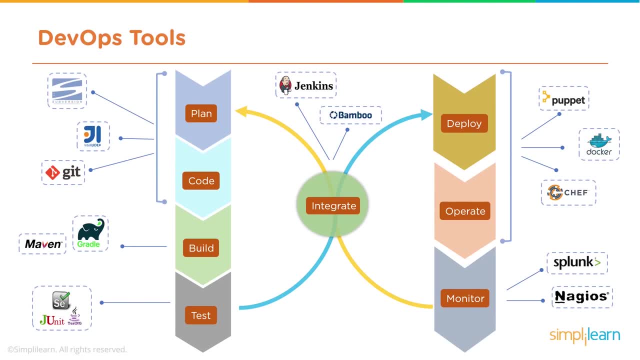 already be using Git, But some of the other tools really help you create a fully scriptable environment so that you can actually start scripting out your entire DevOps tool set. This really helps when it comes to speeding up your delivery, because the more you can actually script out of the 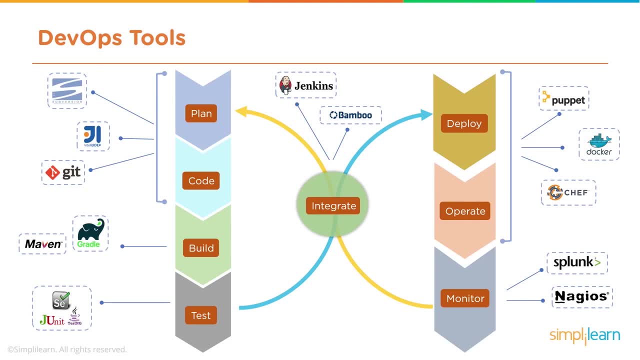 work that you're doing, the more you're going to be able to do the work that you're doing, And so the more effective you can be at running automation against those scripts and the more effective you can be at having a consistent experience. So let's step through this DevOps process. So we go through. 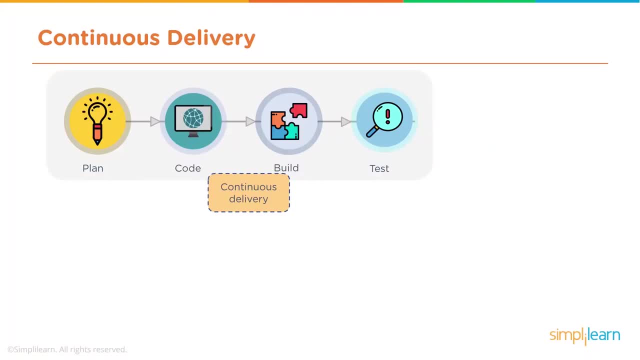 and we have our continuous delivery, which is our plan, code build and test environment. So what happens if you want to make a release? Well, the first thing you want to do is send out your files to the build environment and you want to be able to test the code that you've been created Because 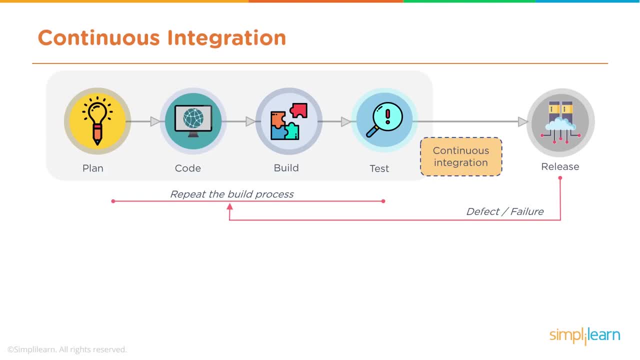 we're scripting everything in our code, from the actual unit testing being done to the all the way through to the production environment. because we're testing all of that, we can very quickly identify whether or not there are any defects within the code. If there are defects, we can. 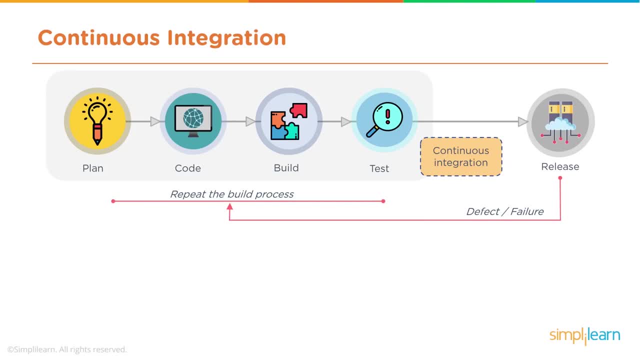 send that code right back to the developer with a message saying what the defect is, and the developer can then fix that with information that is real on the either the code or the production environment. If, however, your code passes the scripting test, it can then be deployed And once. 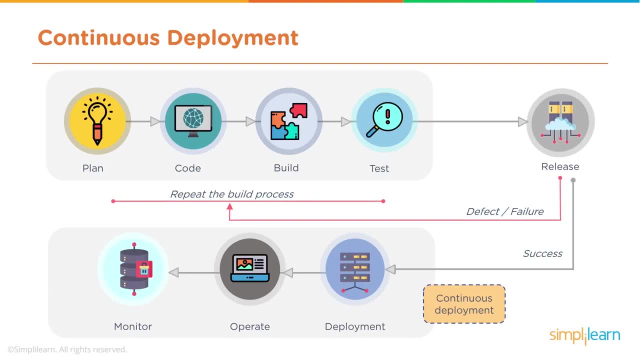 it's out to deployment. you can then start monitoring that environment. What this provides you is the opportunity to speed up your delivery. So you go from the waterfall model, which is weeks, months or even years between releases, to agile, which is two weeks or four weeks depending on your sprint. 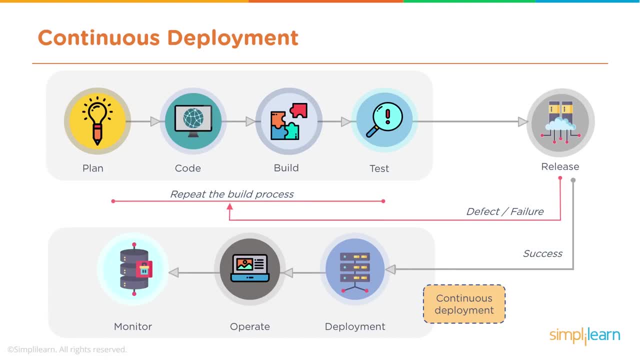 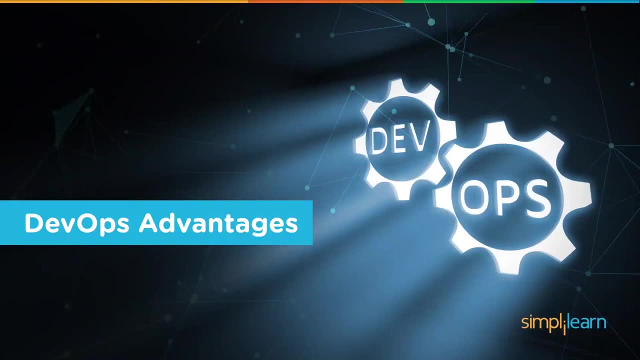 cadence to where you are today, So you can then start monitoring that environment And then you can run the process every single day with DevOps, where you can actually be doing multiple releases every single day. So there are some significant advantages And there are companies out there that are really 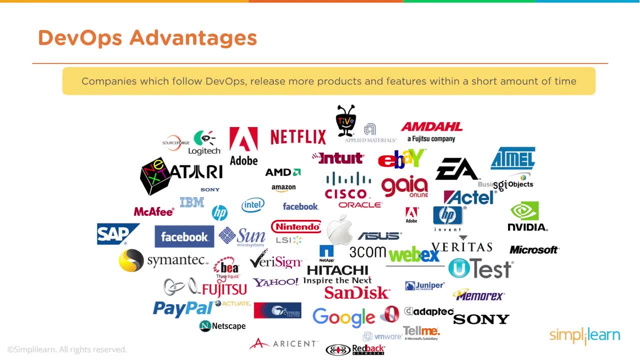 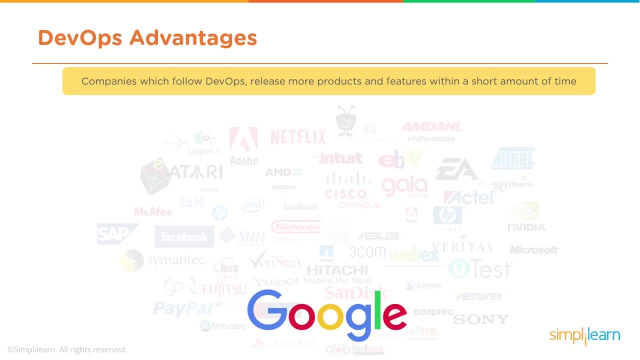 zeroing in on those advantages. If we take any one of these companies, such as Google, Google, any given day, will actually process 50 to 100 new releases on their website through their DevOps teams. In fact, they have some great videos on YouTube. take a look at them And they're going to share those with you so that you can. see them in a few hours. So if you're conscious of what you're doing exactly the same way that you are, you can take a look at them and put a link and go through that and make sure that you're in a room that you need to have. 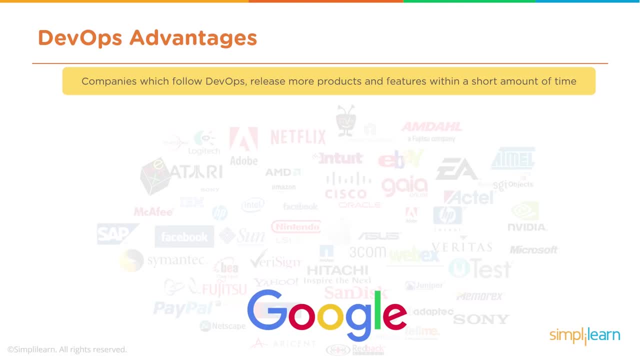 as some basic software with all the tools and all the information, But really what you want to do when you're working on that. you can find out on how their dev op teams work. Netflix is also a similar environment. now what's interesting with Netflix is that Netflix have really 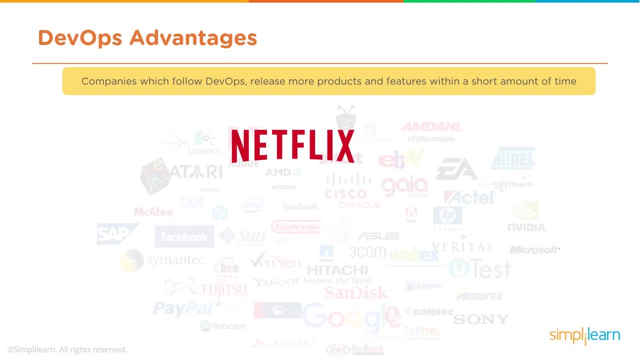 fully embraced DevOps within their development team, and so they have a DevOps team, and Netflix is a completely digital company, so they have software on phones, on smart TVs, on computers and on websites. interestingly, though, the DevOps team for Netflix is only 70 people, and when you consider that, a third of all